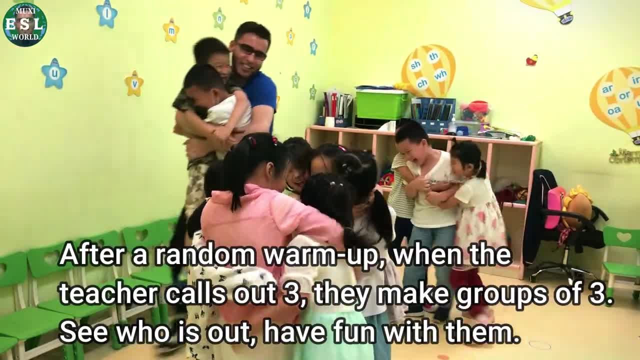 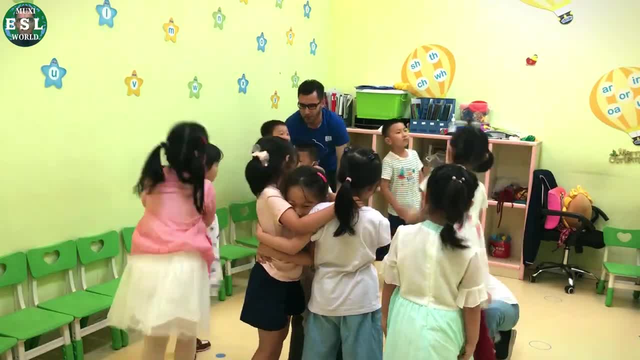 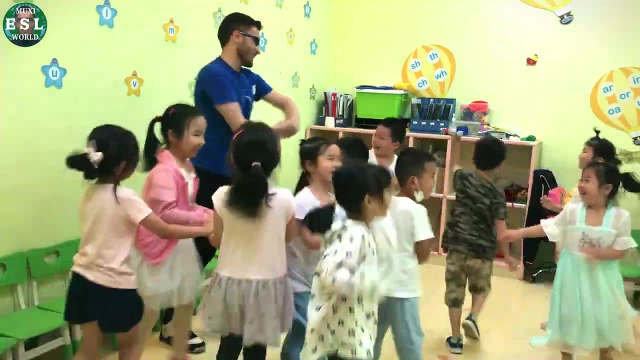 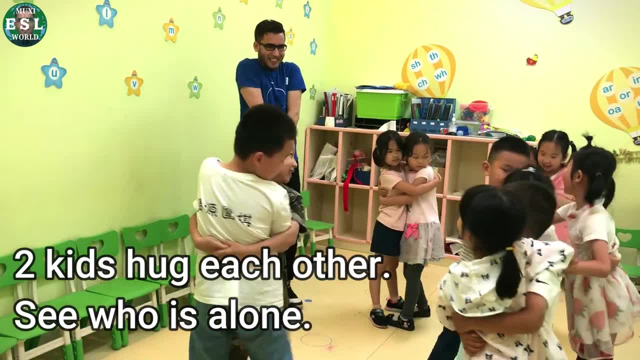 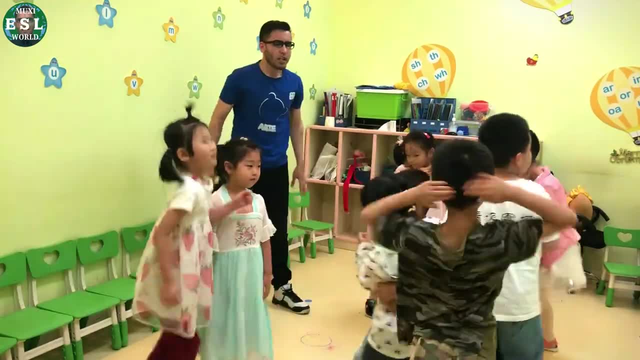 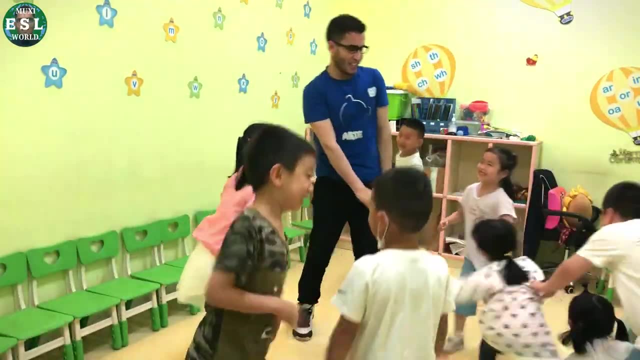 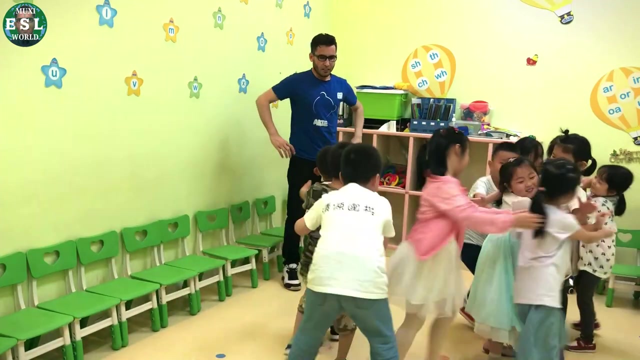 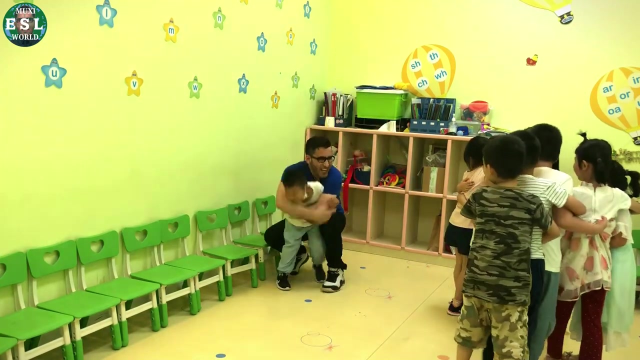 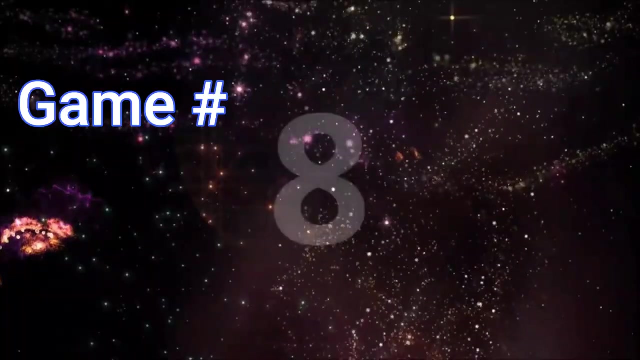 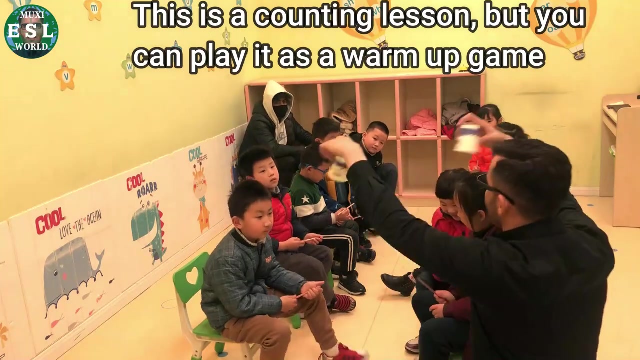 Oh, Jerry's here, Jerry, Jerry, Jerry, Nika. I got Nika Ready, go Five. One, two, three, four, five. I got Jelly. You can pause the cups and put it there on the shelf. We can count later. 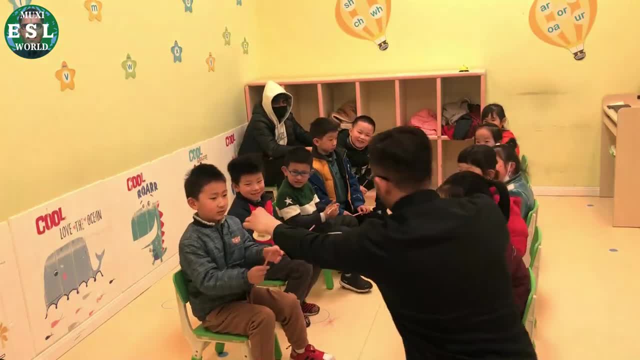 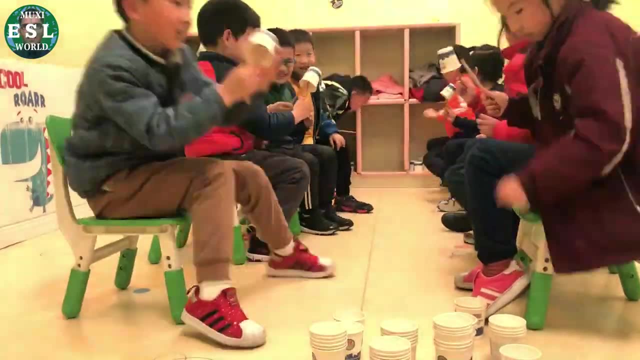 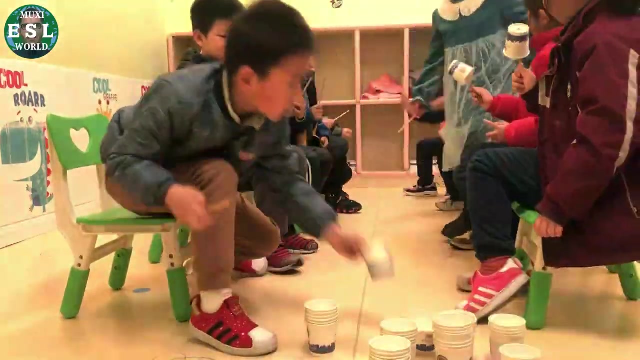 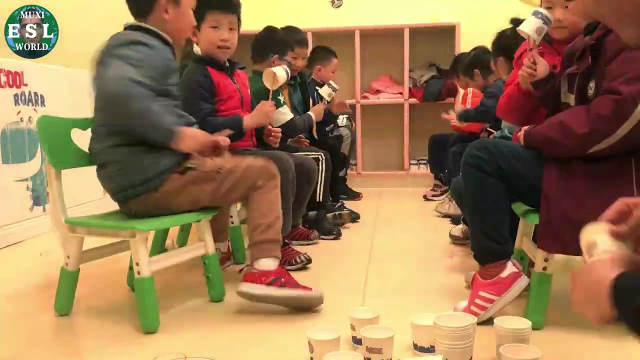 Ready three, two, one whooshie. One hand, one hand only. We are happy. we are happy. we are happy students. We are respectful and we are kind. We value our friends and we value ourselves. We sing, we ask, we sing, we ask. 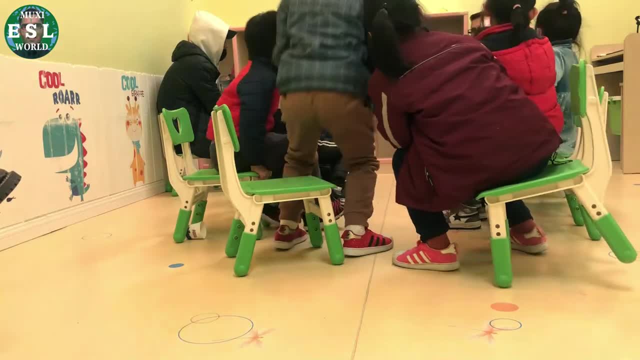 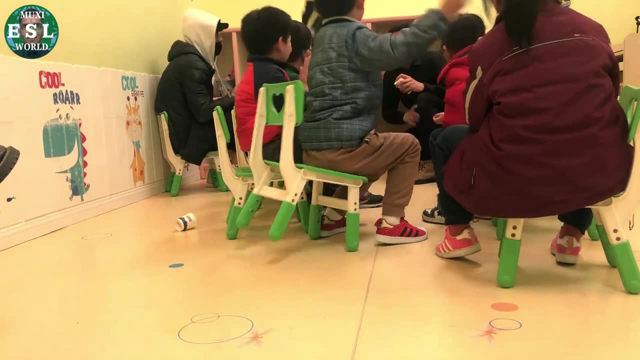 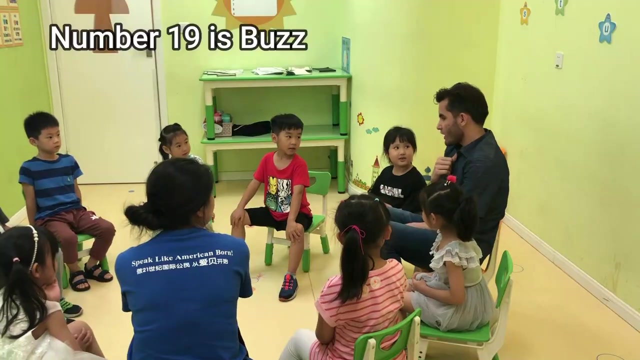 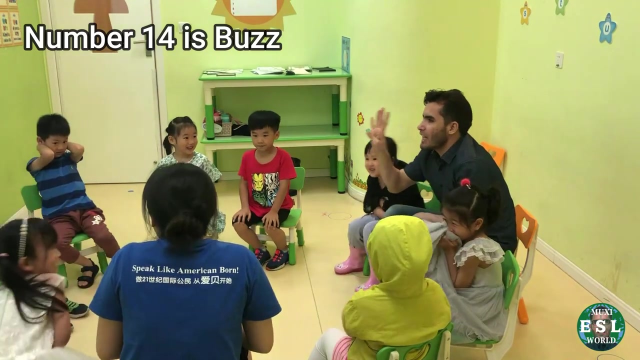 Let's count. Thirty-one to girls. thirty-one, Girls, thirty-one, Thirty-three, thirty-four, Hooray, The boys are the leaders. Seventeen, Nineteen, Nineteen, Fourteen, Ella say one. 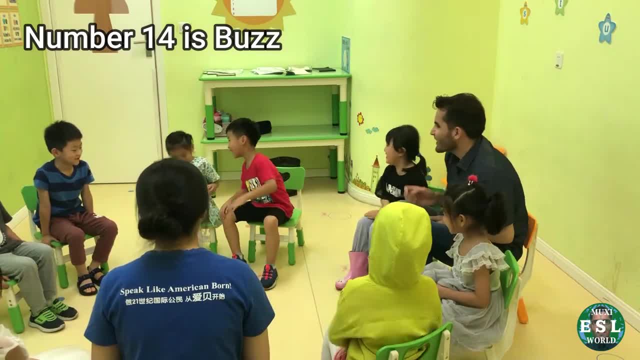 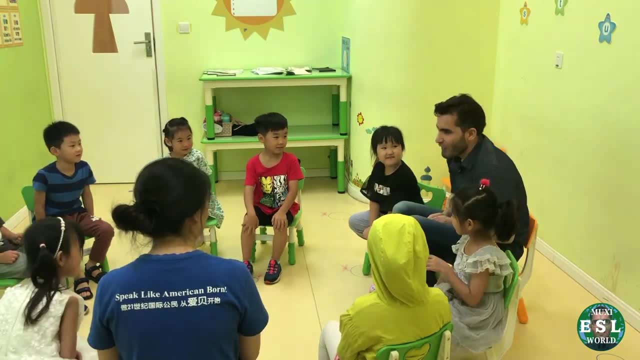 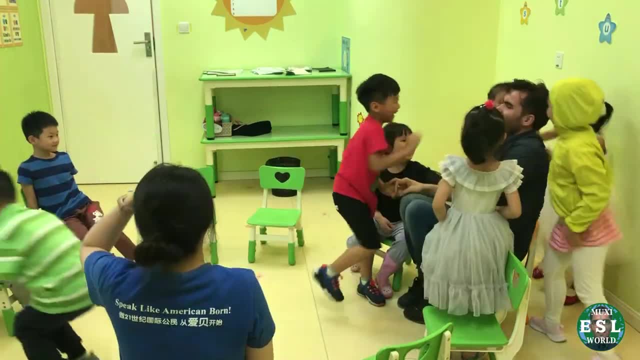 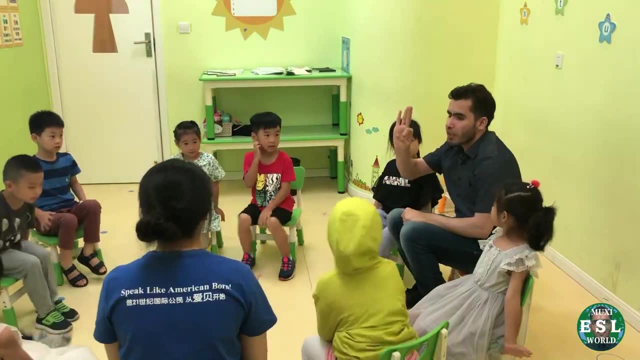 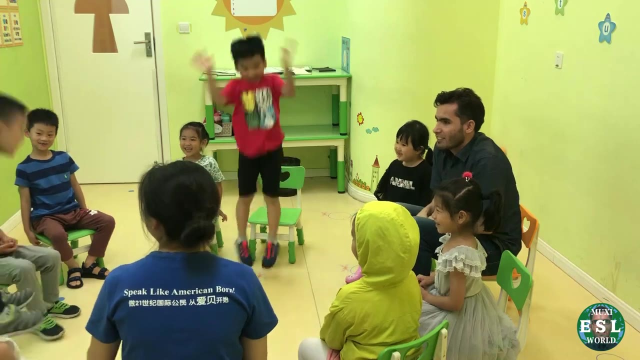 13,, 13, ready One, Two Ready Five, Six, Seven, Eight, Nine, Ten, Eleven, Twelve, Thirteen, Thirteen. Ready One, Two Ready Five, Six, Seven, Eight. 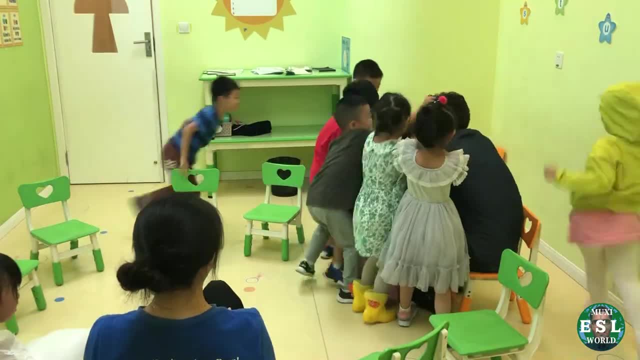 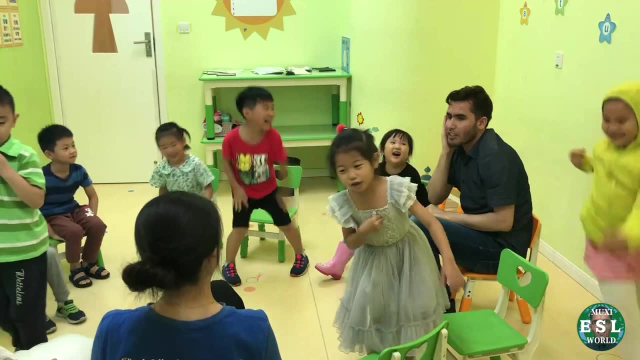 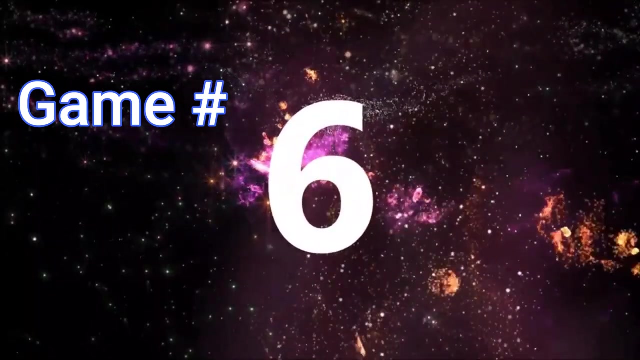 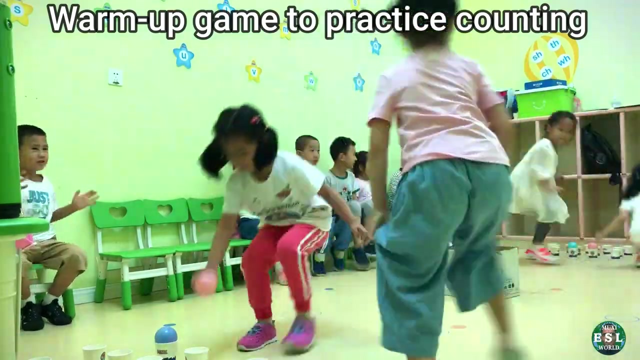 Nine, Ten, Eleven, Twelve, Thirteen, Ten, Twelve One, Three, Five, Four, Three, Two, One. Hurry Ten, Three, Two, One, One… Three, Three, One… Two… Three. 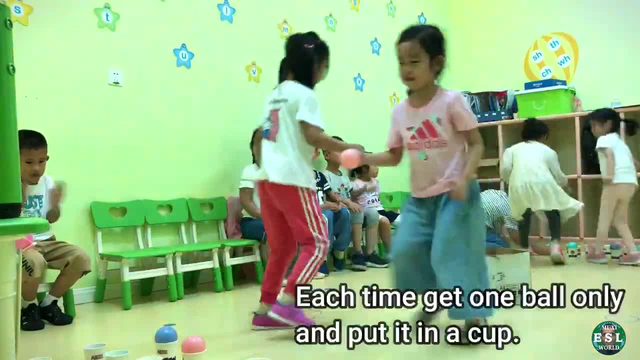 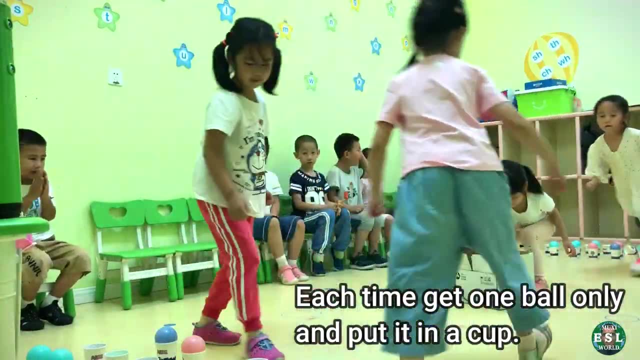 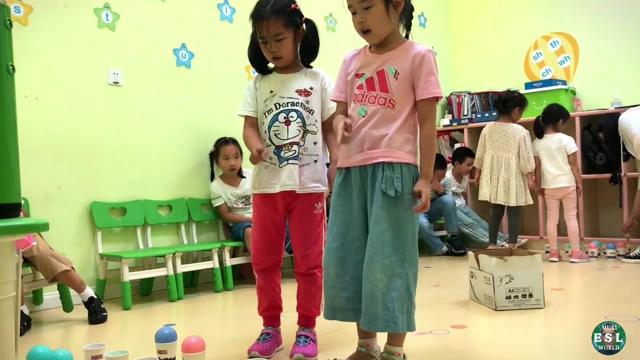 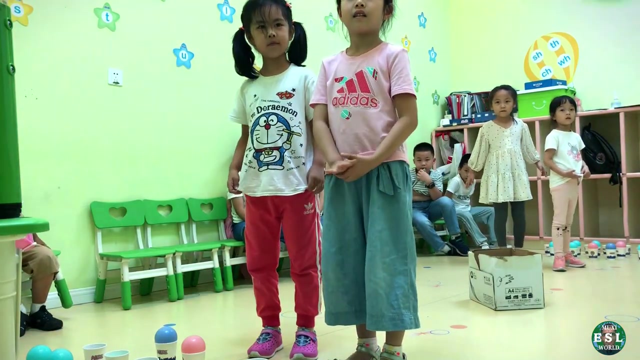 Four Ah, One, Three, Four, Five, Three, One, Two, Five, four, three, two, one, Two, three, four, five, six, seven, eight, nine, 10,, 11,, 12,, 13,, 14,, 15,, 16,, 17,, 17.. 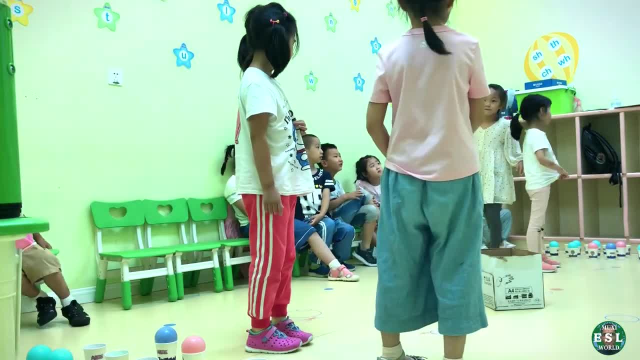 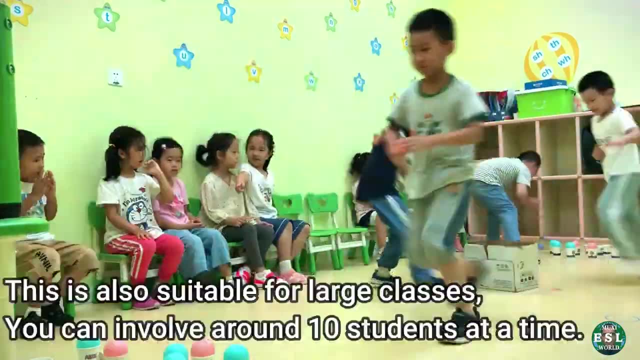 And they got 15.. 15.. They got 15?? Oh, two remaining. Here we go: One, two, three, four, five, six, seven, eight, nine, 10,, 11,, 12,, 13,, 14,, 15,, 16,, 17,. 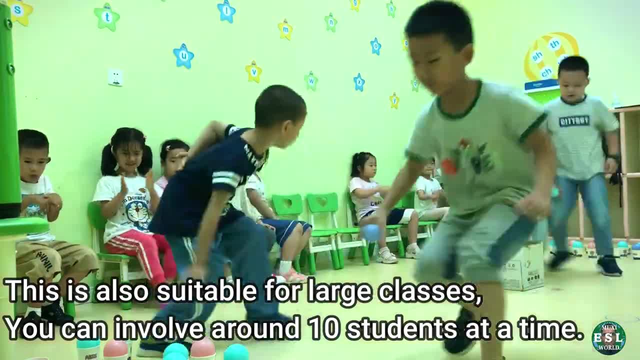 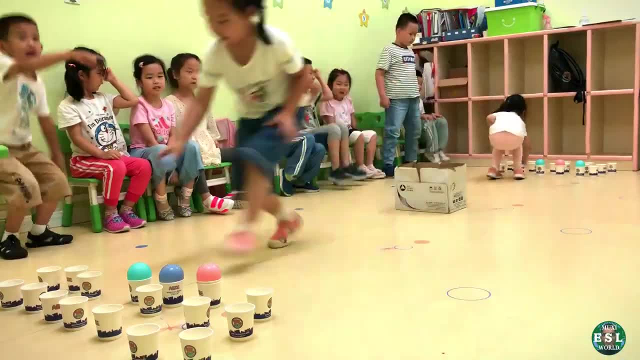 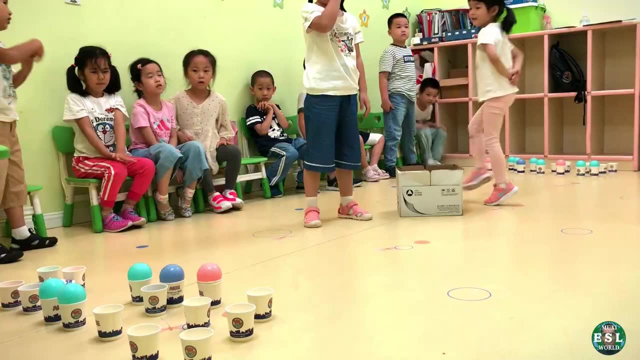 19,, 20,, 21,, 22,, 23,, 24,, 25,, 26,, 27,, 28,, 29,, 30.. One, two, three, four, five, six, seven, eight, nine, 10,, 11,, 12,, 13,, 14,, 16,, 17,, 18,. 29,, 20,, 21,, 22,, 23,, 24,, 25,, 26,, 27,, 28,, 29,, 30. 15.. 15.. How much $15.. Thank you. 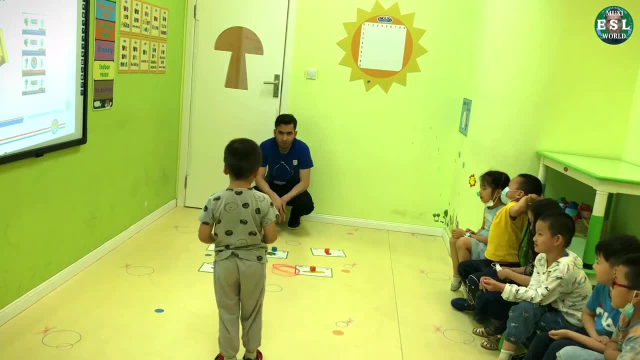 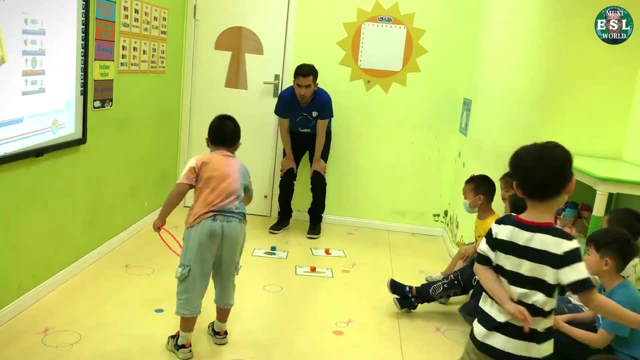 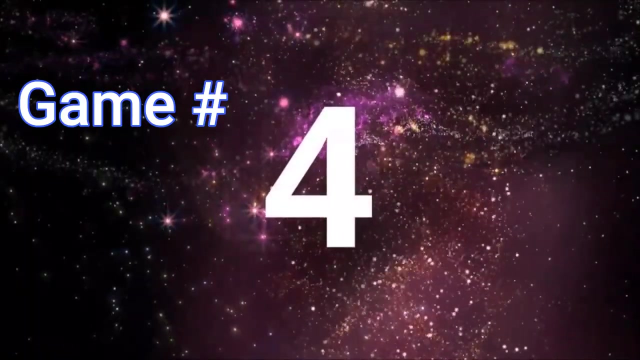 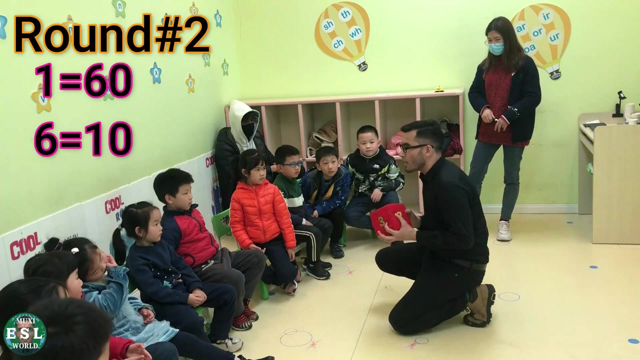 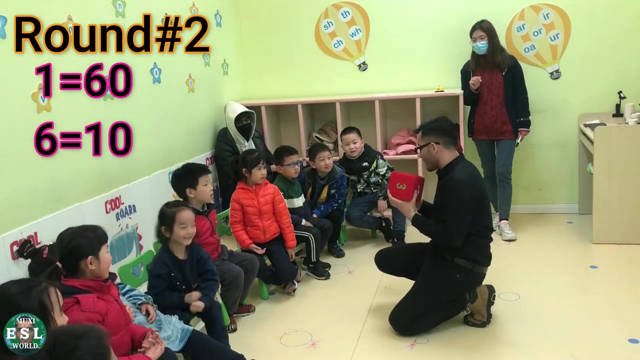 How much, How much, How much? If you got 5,, you get 50.. If you got 3,, you get 30. But if you got 1,, you will get 60 points. If you got 6,, you will get 10 points. 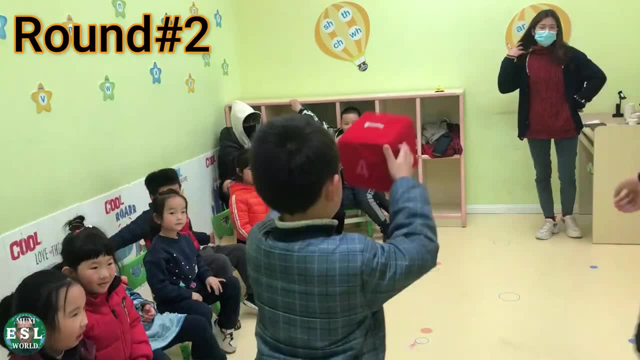 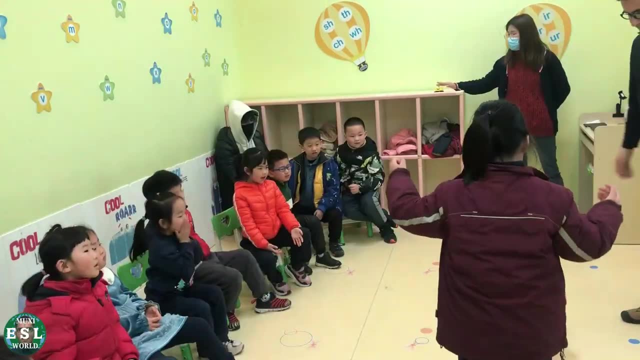 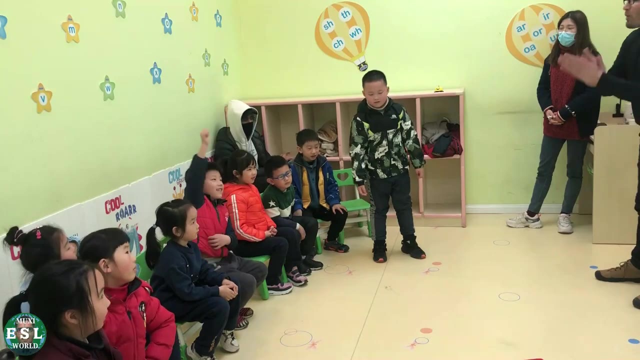 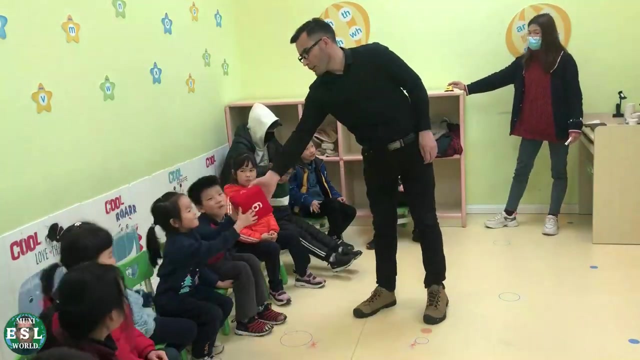 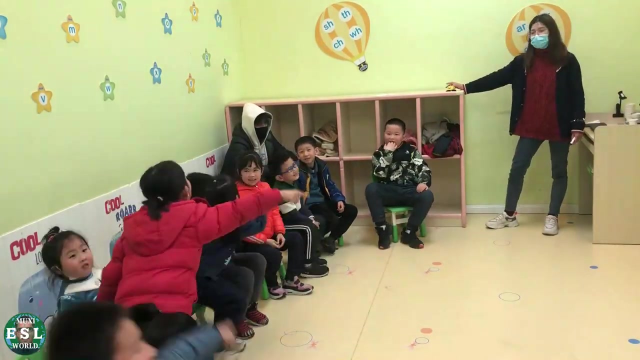 Yes, sir, Ready Go Jim's turn Jim go. 60 points. You got 6, so you get 60 points. 30 points. So let's count Boys 90.. Ah, I'm okay, I'm okay. 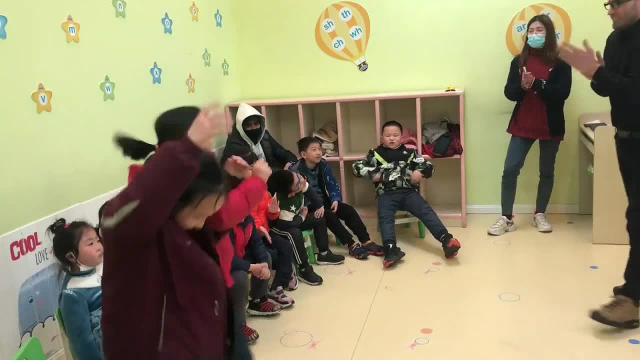 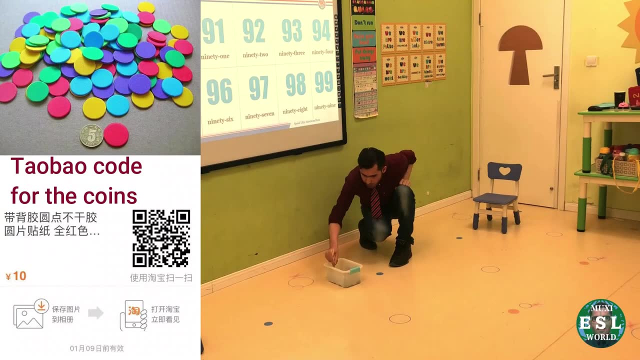 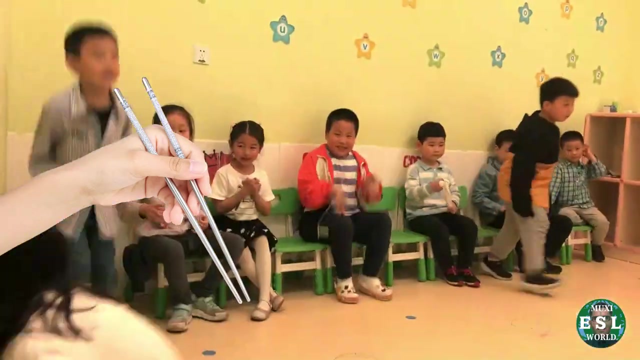 So girls are the winners. So you got to use chopstick. Pick up one right, put it on the chair and give the chopstick to the next person. We are happy, we are happy, we are happy students, We are respectful and we are kind. 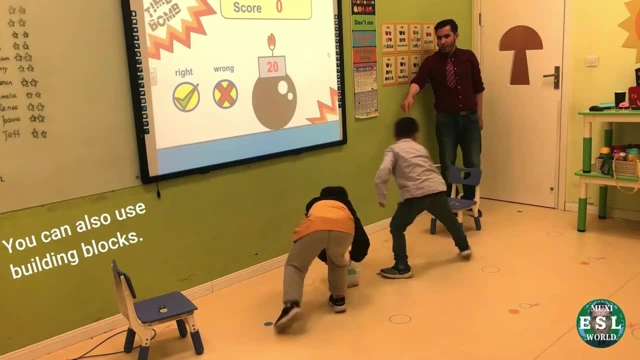 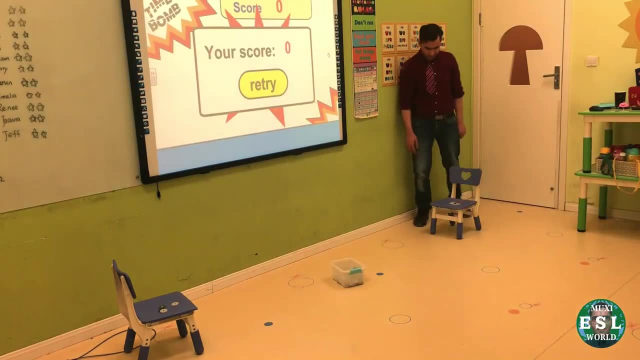 We value our friends and we value ourselves. We are the success of commercials. Uh oh, let's count. We are the success of commercials 1,, 2,, 3,, 4,, 5,, 6,, 7.. 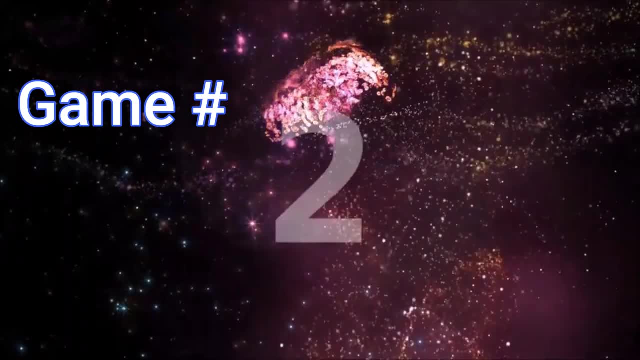 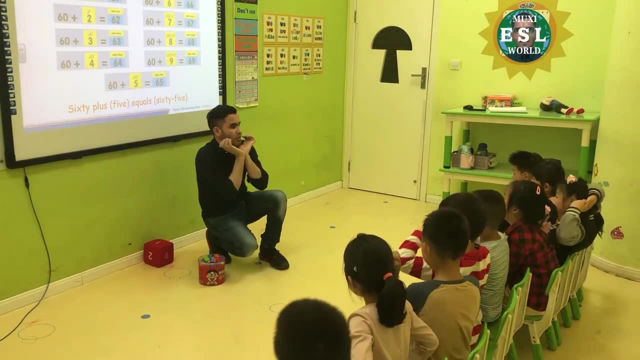 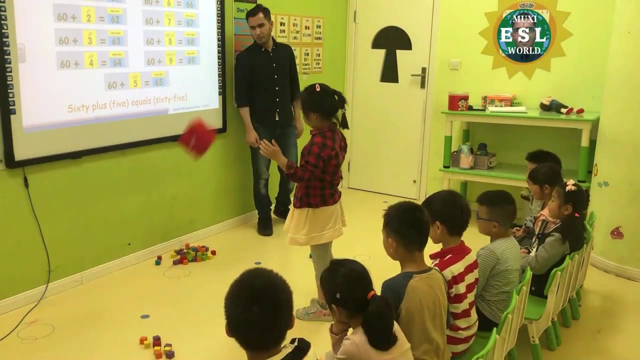 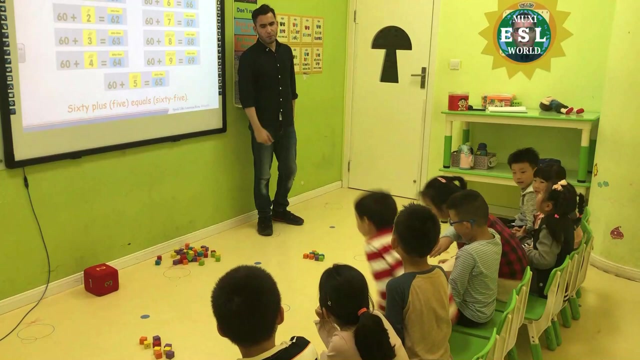 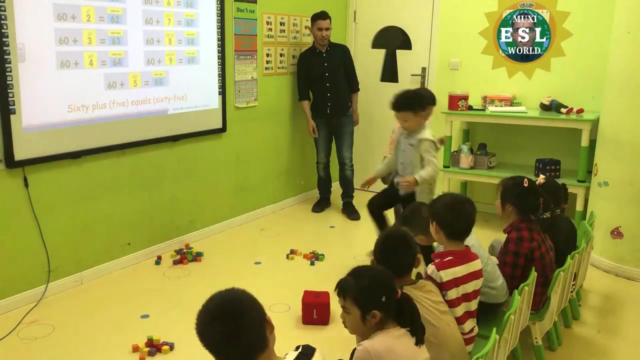 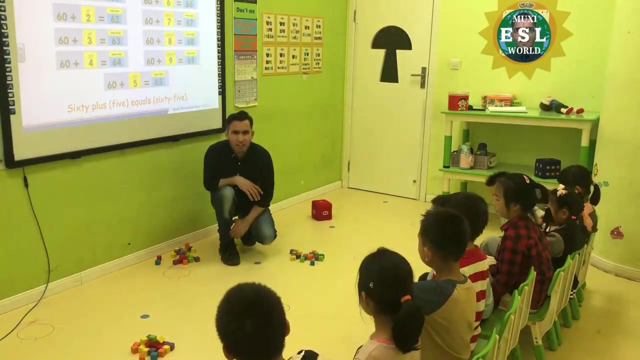 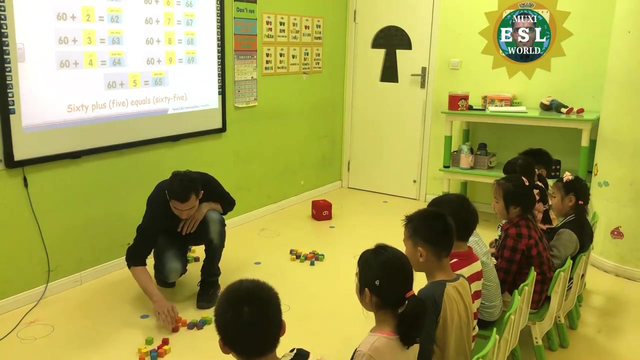 1,, 2,, 3,, 4.. crucifix of technology. We have two teams, boys and girls, four, two ah two. One, two, three, four, five, six, seven, eight, nine, 10,, 11,, 12,, 13,, 14,, 15,, 16,, 17,, 18,. 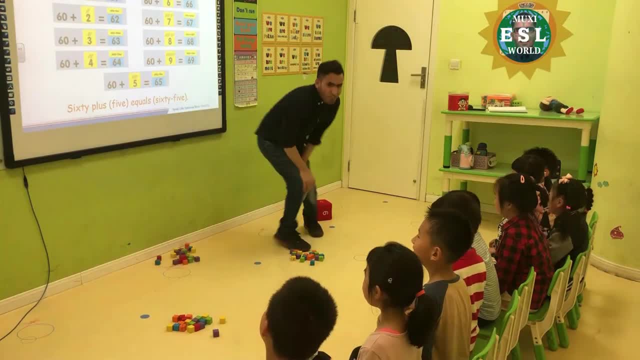 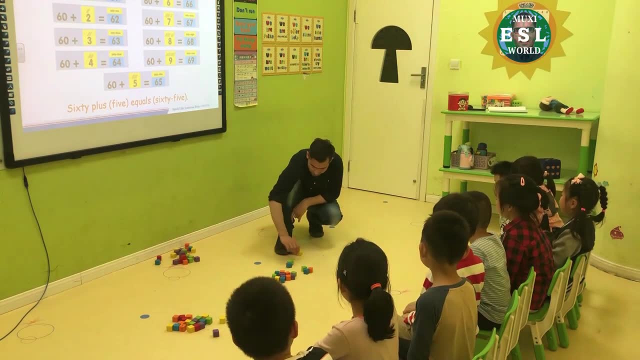 19, 20.. Girls One, two, three, four, five, six, seven, eight, nine, 10,, 11,, 13,, 14,, 15,, 16,, 17,, 18,, 19!. 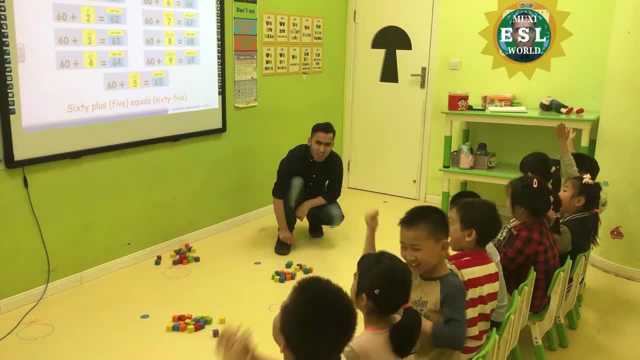 Just one point: Team one boys, Team two girls. You're gonna roll the dice: If you get five, you will get 50.. If you get five, you will get 50. You can do it, You can do it.